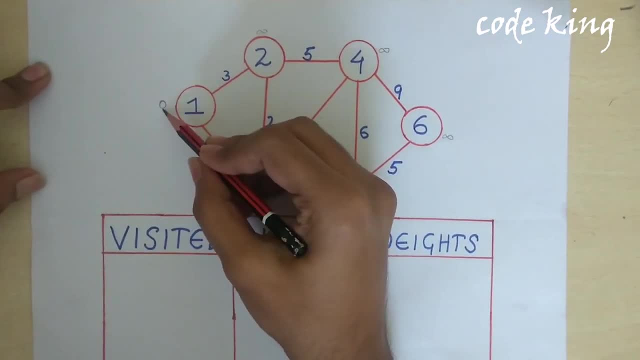 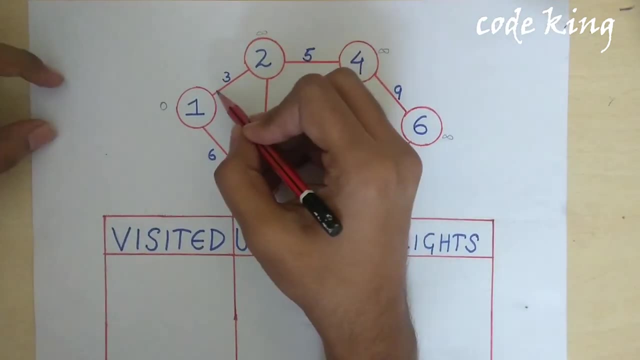 node 0. The weight of the source node is 0 and all the other nodes are infinity. The weight represent the distance from the source node and the edge weight is given. So now let's mark the source to be visited, for now. 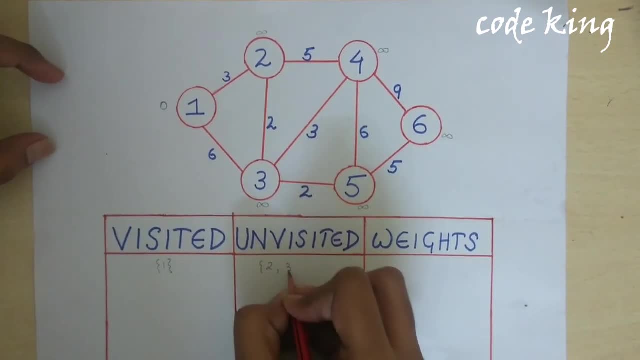 And write the unvisited. The unvisited nodes are here: 2, 3,, 4,, 5, 6.. All these nodes are unvisited and the weights associated with them are 0.. The weight for the node 1 is 0.. For node 2, it's infinity. 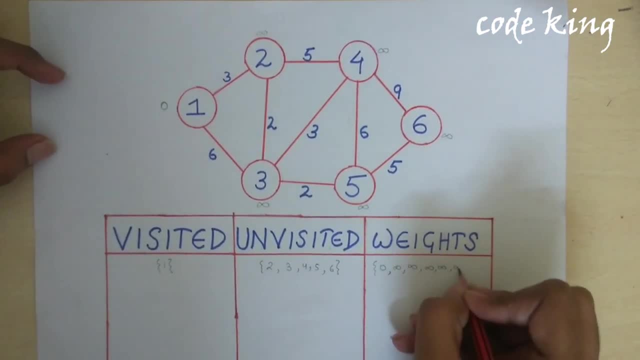 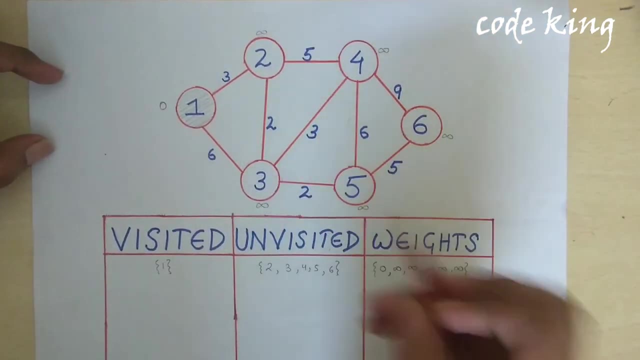 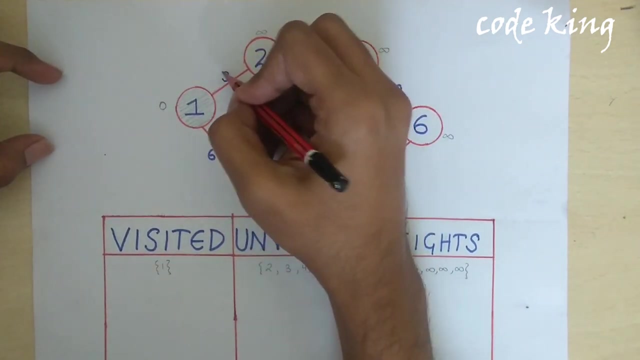 For node 3, it's infinity, And for all the other nodes it's infinity. as we can see Now we have marked it visited, so we are shading it just for the sake of clarity. Now we are going to this. So the distance is 3.. 0 plus 3 is 3.. Since it is less than infinity, we are going to. 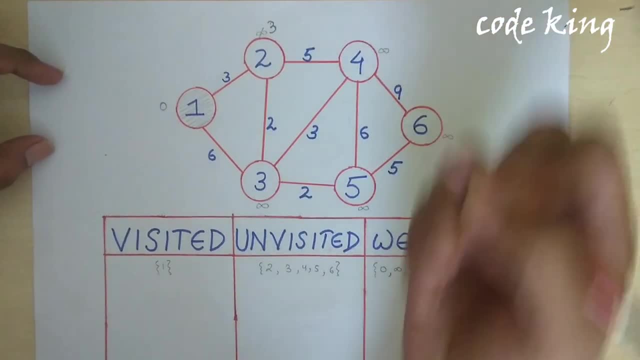 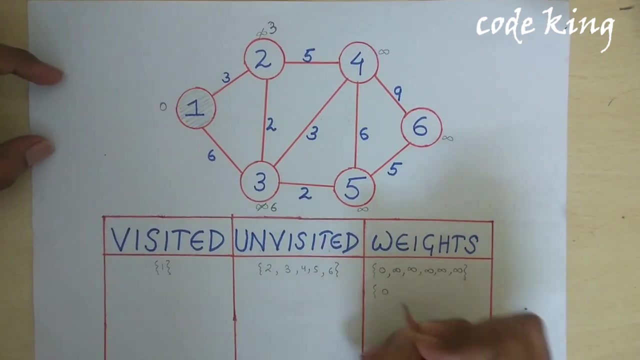 update the distance, the weight of the node. It is 3.. And for here it is 0 plus 6 is less than infinity, it is 6.. Now we are going to update it. So the new weights are 0,, 3,, 6,. 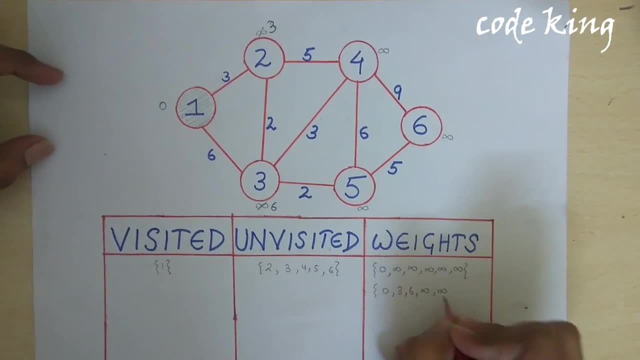 infinity, infinity, infinity. and now we are going to take the node which is having the minimum weight out of the unvisited nodes. so the weight for the second node is 3 and the third node is 6 and for rest it's infinity. so the minimum weight is 3, associated with the 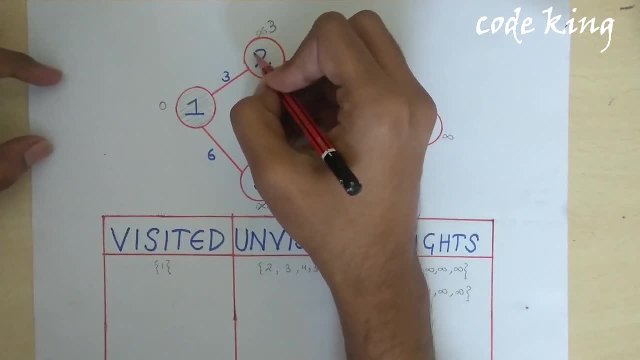 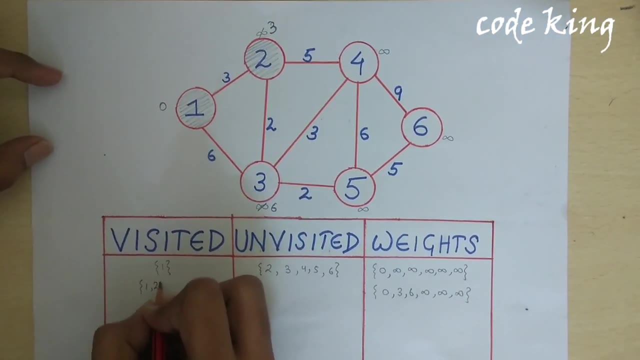 second node. so we are going to take the node 2 into consideration and mark it visited. we are marking it visited and the unvisited nodes that remains are it's 5. so now exploring all the neighbors of the second node. remember, we are going to explore only the neighbors which are unvisited, not the 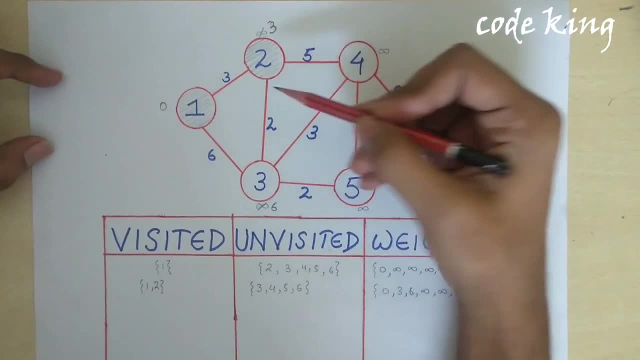 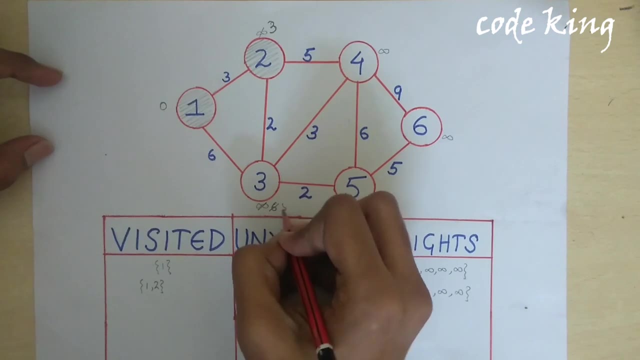 unvisited ones. so the ones which are unvisited and directly connected to the node 2 are node 3. it's 3 plus 2 is less than 6- 6, so we are going to update it. 3 plus 5- 8- less than infinity, so we are going to update. 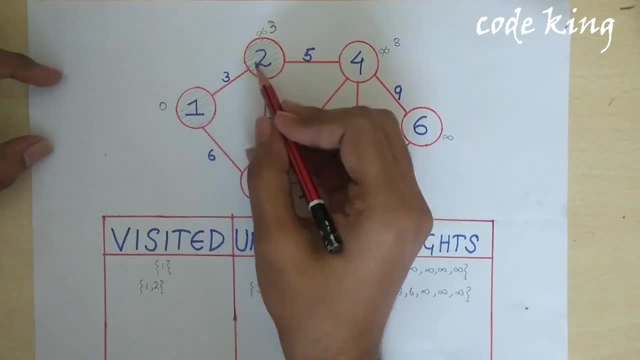 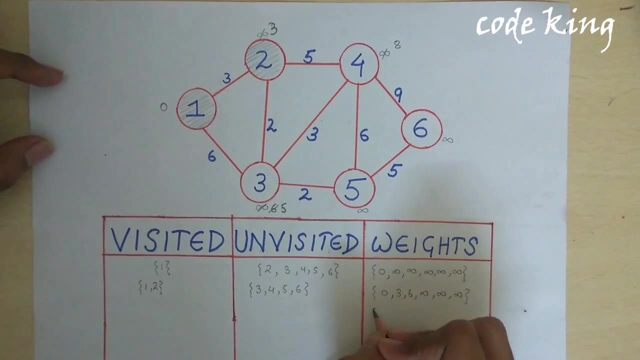 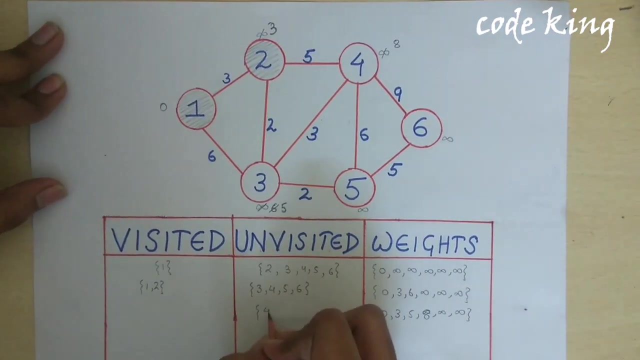 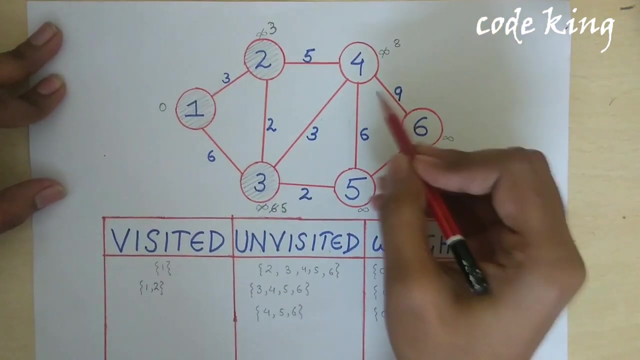 it. so we are not going to update the weight of this because it's already revisited. so now the new weights are 0, 3, 5 and 8, infinity, infinity. the remaining unvisited nodes are 4, 5, 6, because we are going to mark it visited, since from the remaining nodes it's having. 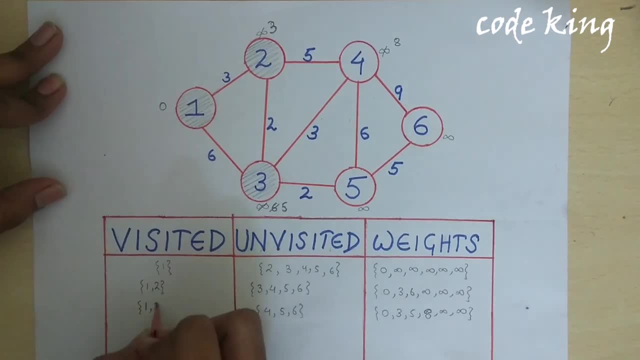 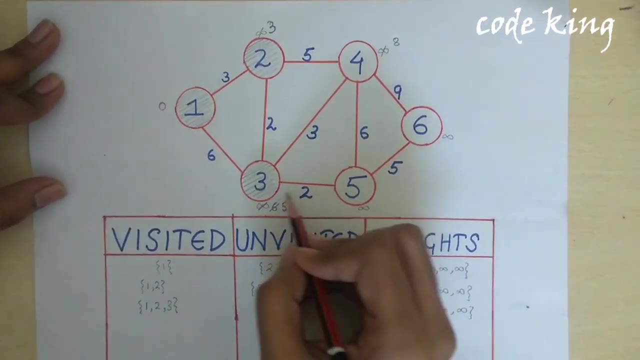 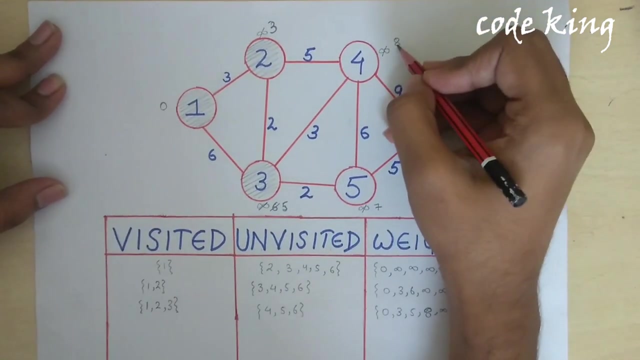 the minimum weight: 1, 2, 3, and we're going to explore its neighbors. so its neighbor is 5. 5 plus 2 is 7, less than infinity. 5 plus 3 is equal to 8, so it's 8. we are not going to. 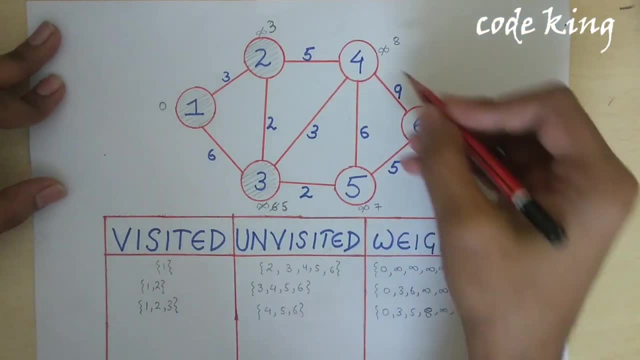 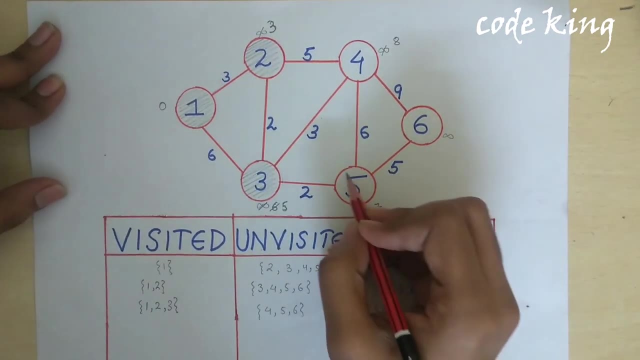 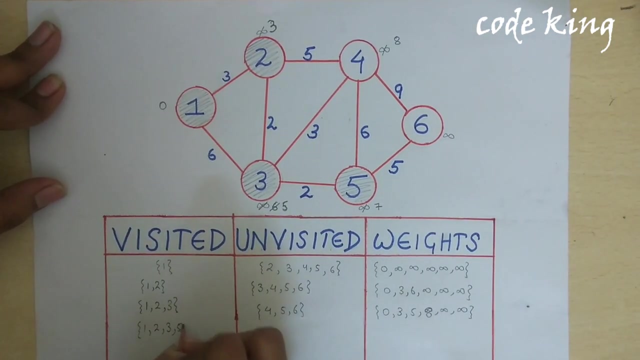 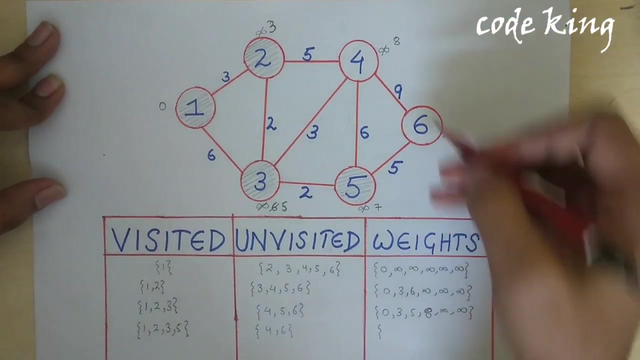 update it: it's already 8 and from the rest of the nodes, 5 is having the minimum weight, so we are going to mark it visited now 1, 2, 3, 5. weight remaining are 4 and 6, the weights associated with them. 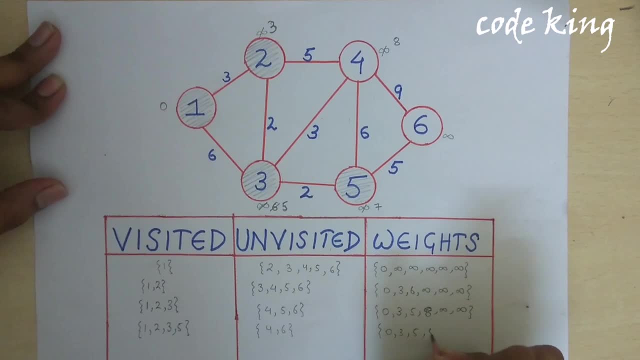 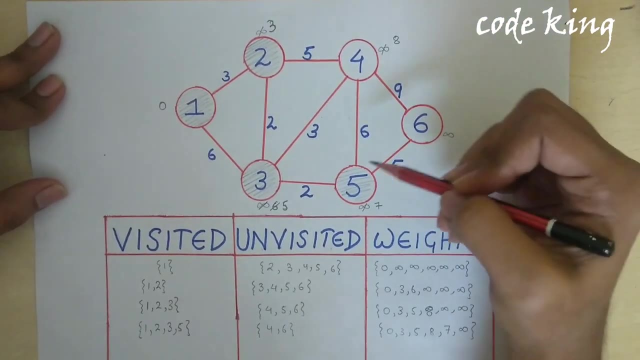 are 0, 3, 5, 8, 7 and infinity, so we are going to explore its neighbors. 7 plus 6, it's 13, it's more than 8, so we are not going to update it. 7 plus 5, it's 12, it's less than infinity. so we are. 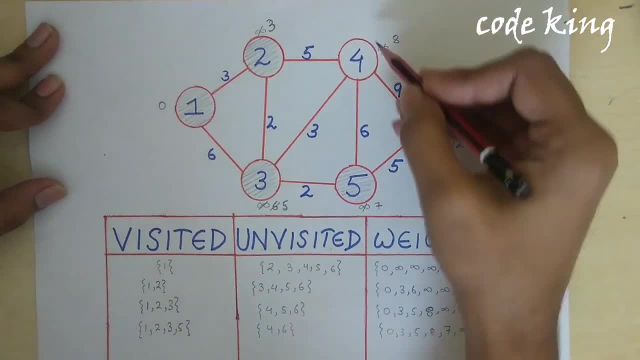 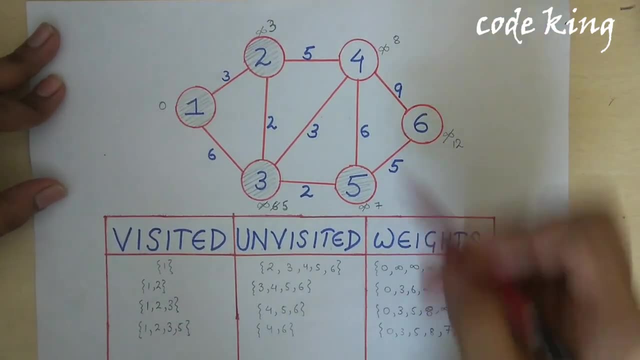 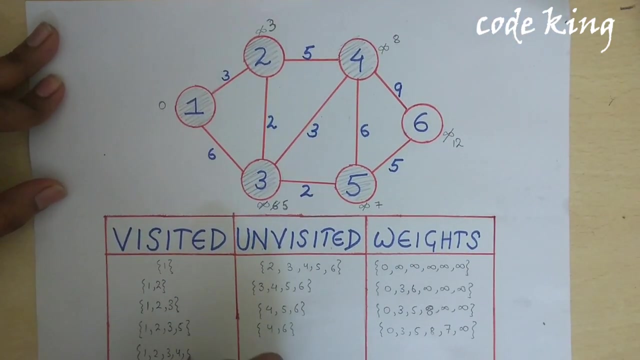 going to update it and from the remaining nodes, it's clear that we are going to take node 4 into consideration, since its weight is minimum out of the unvisited nodes, and we are going to mark it: visited: 1, 2, 3, 4, 5. all these nodes are visited and only 6 remains, the weight associated with. 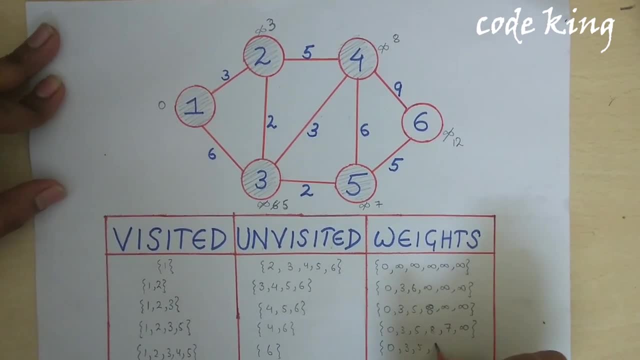 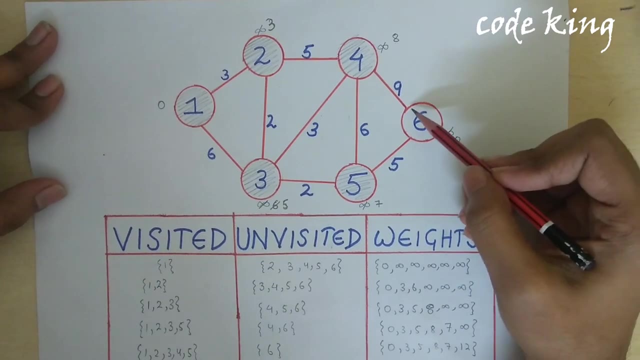 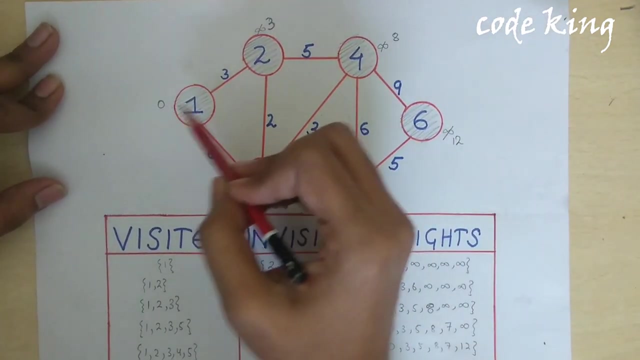 them are 6, 3, 5, 8, 7 and 12. now only 6 remains and all the other nodes are unvisited. so we are going to mark it visited and we are not going to change the weight. so now, as we clearly see, 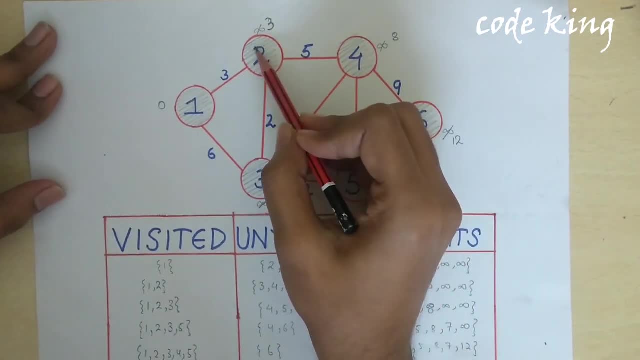 node 1. we have calculated the minimum path possible to all the other nodes. thank you for the same.